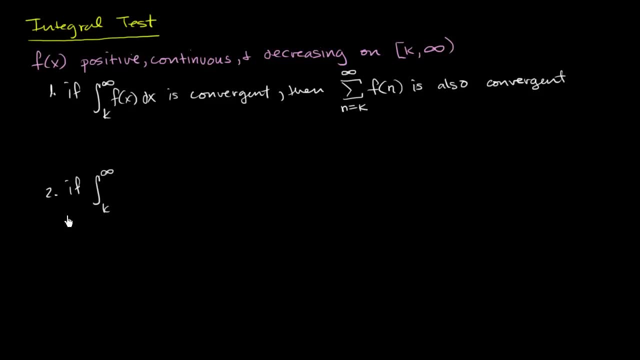 That if the integral from k to infinity, the improper integral of f, of x, dx, is divergent- divergent, then the same thing is true for the corresponding infinite series, Then this infinite series right over here is also going to be, is also divergent. 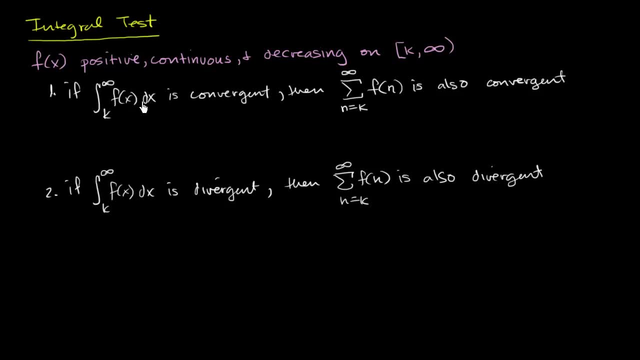 And, as I already mentioned in the last video, we already saw this in the case of f of x is equal to one over x squared. We saw that since the integral from one to infinity of one over x squared Over one over x squared, dx is convergent. 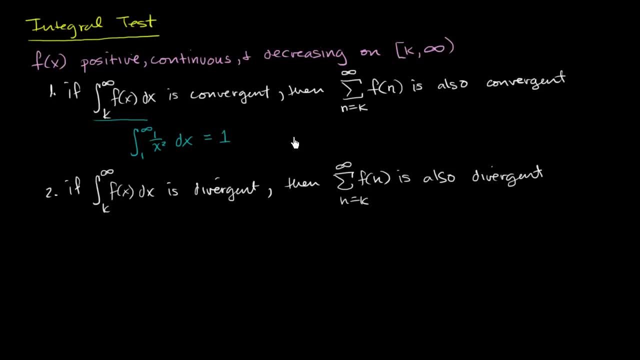 In fact it equals one. It equals one. Because of that, we were able to say that the sum from n is equal to one, to infinity of one over n squared is also convergent. And now we can see an example where we go the other way. 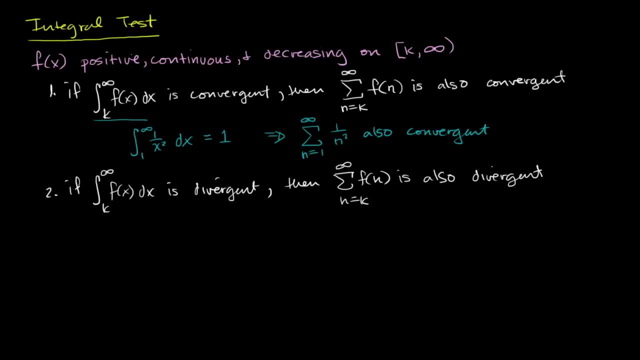 For example, we know that this integral- let me write the integral down. let's start with this integral From one to infinity, not of f of x- is equal to one over x squared, but let's say that f of x is equal to one over x. 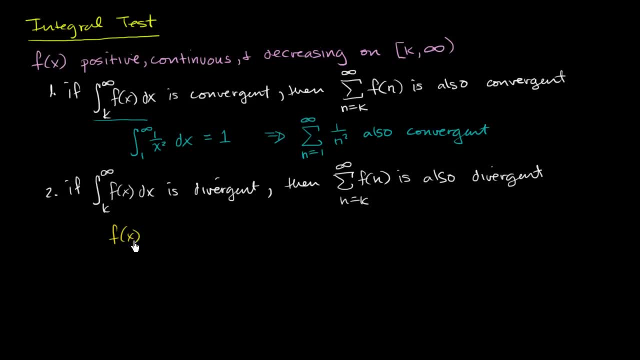 Actually, let me just write that down. Let's just start with: f of x is equal to one over x. It definitely meets our conditions that it is positive. and let's say we're gonna consider it over the interval, over the interval from one. 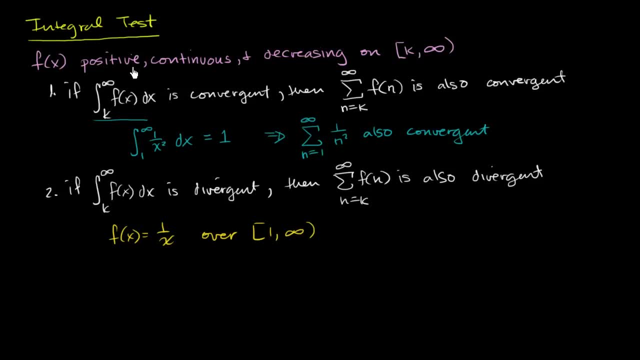 to infinity. So it meets this first constraint. Over this interval, one over x is positive, it is continuous and it is decreasing. As x increases, f of x decreases. So the integral test should apply. So let's see what the improper integral 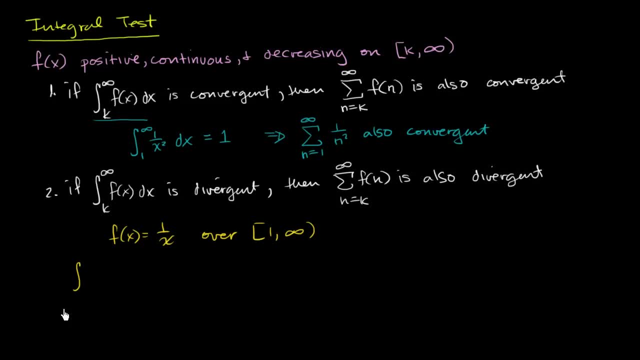 from one to infinity of this would be So, if we go from one to infinity, of one over x, of one over x, dx, this is equal to: we could write this as the limit as t approaches infinity of the definite integral: from one to t. 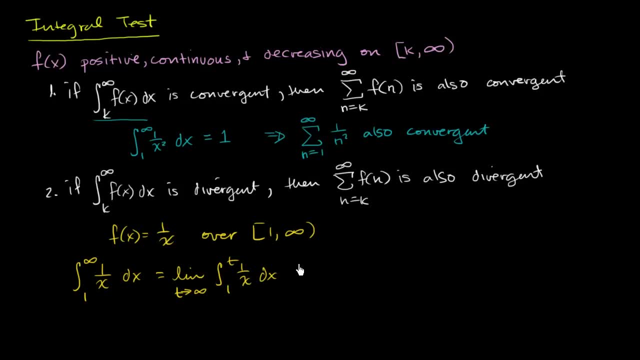 of one over x dx, which is equal to the limit, as t approaches infinity, of take, the antiderivative is going to be of the natural log of x, the natural log of x, the natural log of x going from one to t. 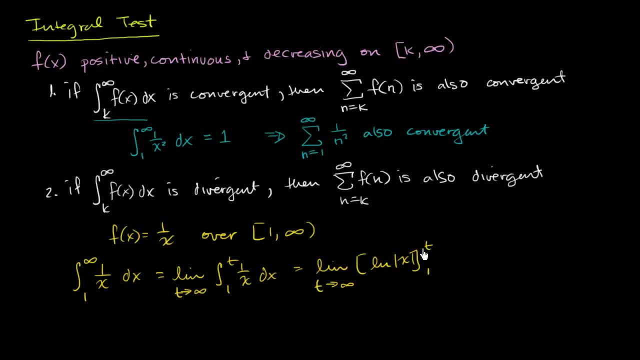 one to t. we could do the well. it's really the absolute value of x, but we're dealing with positive x's here, so it's just going to be the natural log of x which is going to be the limit as t approaches infinity. 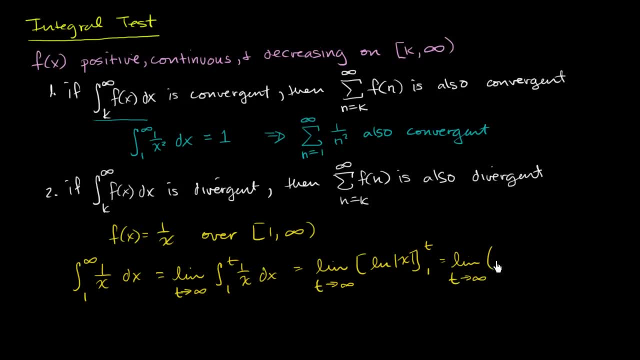 of the natural log of t, or I could even say the natural log of the absolute value of t, which is just going to be the natural log of t because it's positive t's minus the natural log of one, minus the natural log of the absolute value of one. 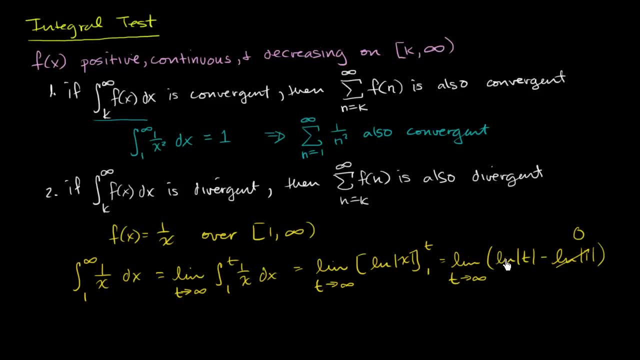 Well, the natural log of one is zero, so it's going to be the natural log of t, the limit as that approaches infinity. but the limit as that approaches infinity is just going to be unbounded. This is going to go to infinity. 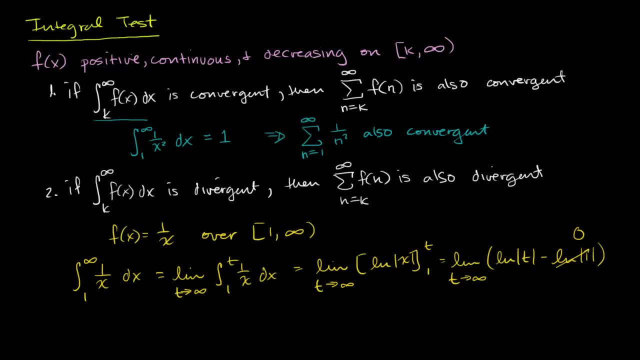 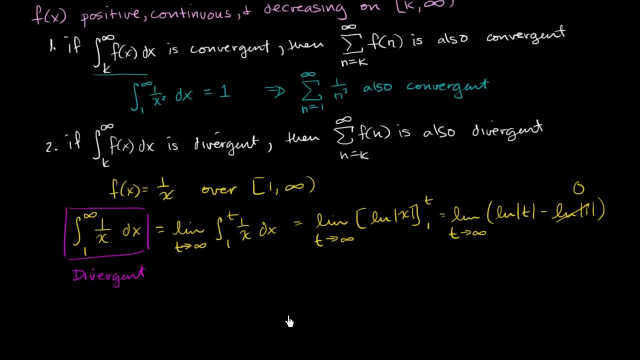 This right over here is divergent, so this right over here is divergent, So this is divergent. And because this is divergent, we can then say, we can then say: by the integral test, we can then say the integral test. 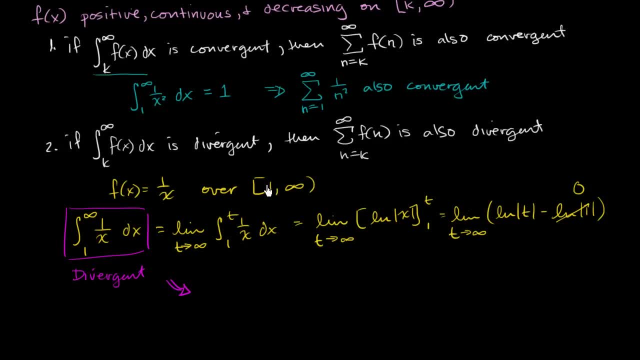 once again our function over this interval positive, continuous decreasing. we saw that this improper integral right over here is divergent. and then by the second point of the integral test, we can say therefore- and I haven't rigorously proved it yet- 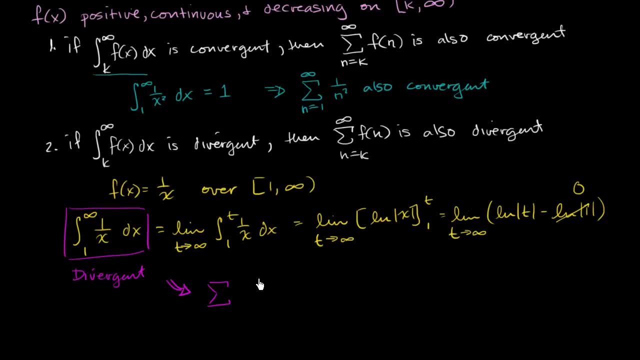 but hopefully I gave you a good intuitive justification in the previous video that the integral, that the infinite series from n equals one to infinity of one over n, which is the harmonic series that this is also. this is also. this is also divergent. 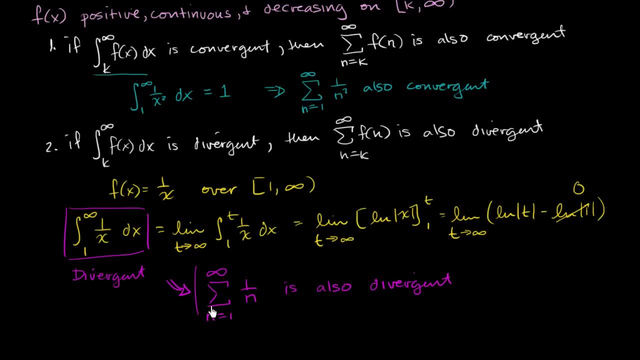 So we've already shown that the harmonic series is divergent using that very beautiful, elegant proof by Orem- I think I'm probably mispronouncing his name- that used the comparison test, but just like this, we have used the integral test. 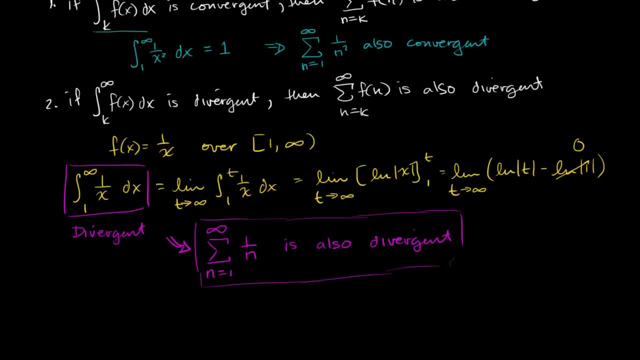 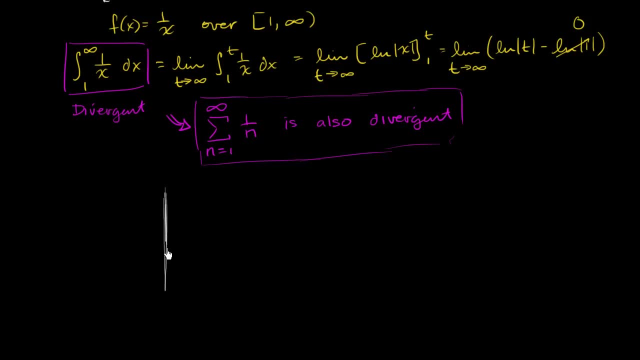 to show that it is also divergent. And once again, let's remember what the whole motivation of the integral test is. Let me draw: f of x is equal to one over x. So f of x is equal to one over x, would look like. 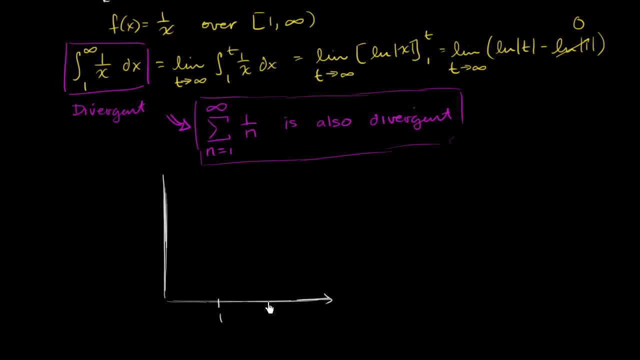 do my best attempt here. so let's say: that's one, two, three, that is one, two. and so let's see: when x is one, f of x is one. when x is two, f of x is one half. 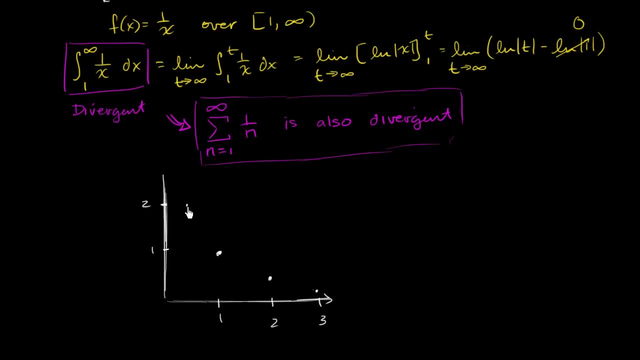 one third, that's one half here. it'll be two over here, so it looks like this: So this is f of x is equal to one over n, and once again we see that over the interval we care about, from one to infinity. 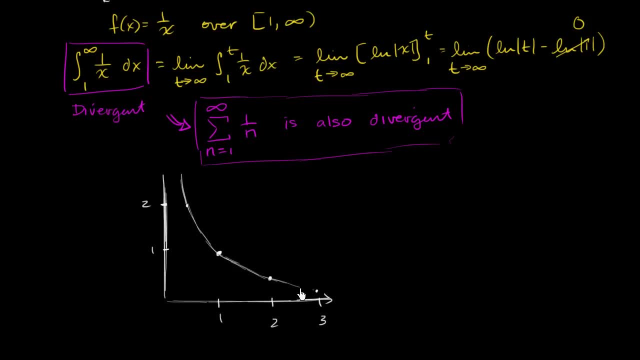 it's definitely positive, continuous and decreasing, And if we look at this sum right over here, we could view this sum as. let's do that. let me write it down. So the sum, the sum from n, equals one to infinity. 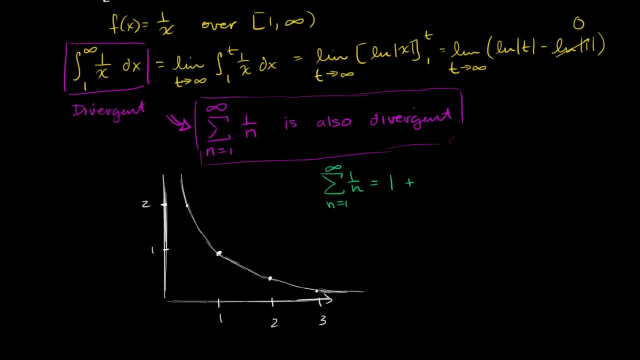 of one over n is equal to one plus one half plus one third, and of course we keep going on and on, and on and on. In this case, since we want to show this divergent, we could say: hey look, this is an overestimate. 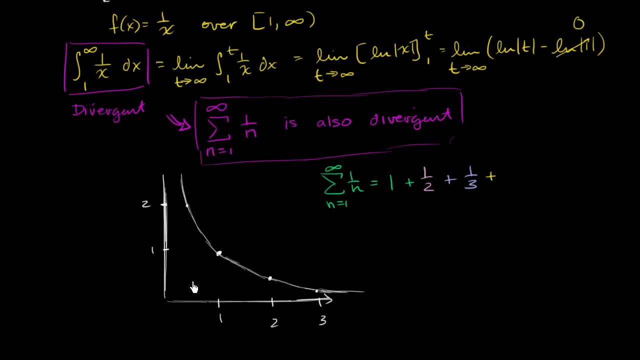 of this area here. let me be clear: So we have this area, we have this area in green, which is what the improper integral is denoting, so that right over there is the improper integral from one to infinity of one, over x, dx. 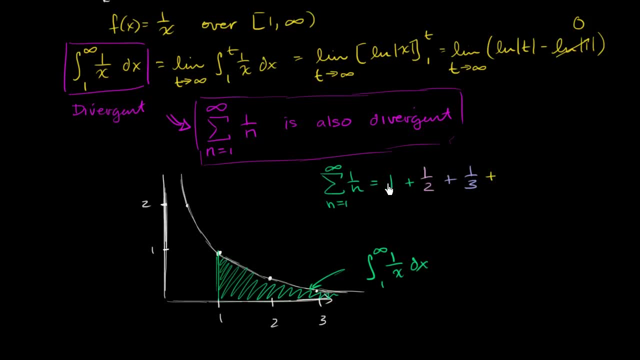 Now you could view this as an overestimate of that area. So this first, this one right over here, you could say that this is this one height times one width. so that's that block right over there, that's the area of that.